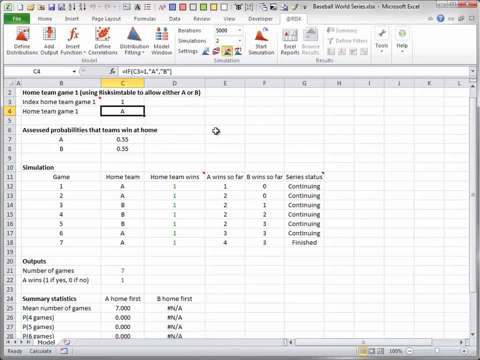 For now, the model assumes that the two teams are going to win two games. That's the first one, The two teams are equally good and that each has probability 0.55 of winning in its home stadium. Of course, these probabilities in rows 7 and 8 can be changed to any values you like. 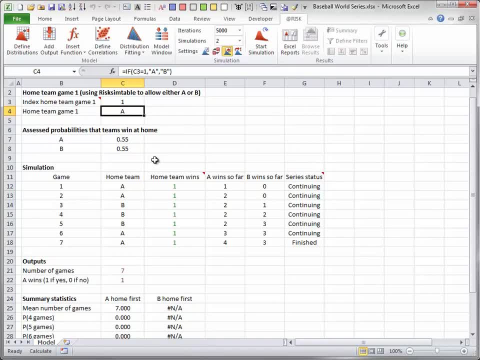 But with the current assumption of equally good teams, you would probably expect that the team with first home field advantage should have an edge in the series. right After all, this team will play a potential four games at its home stadium, whereas the other team can play at most three games. 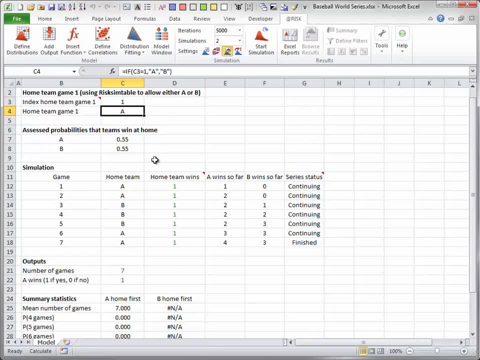 The simulation will eventually indicate how much of an edge there is. Note that the at-risk dice button is currently set to static values For this model. it is more interesting to change this to random so that you can see how different iterations of the series can play out. 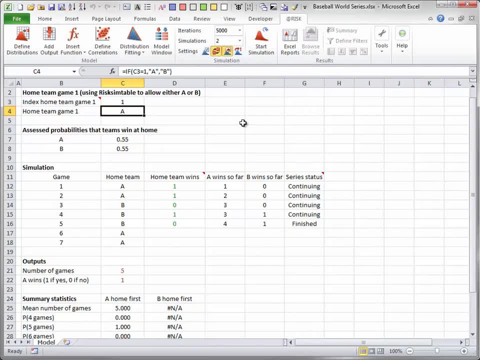 The simulation itself is a little tricky, because the Excel formulas have to capture two types of logic. First, they have to indicate which team is the home team in each game, and second, they have to indicate when the series is over. Here is how this logic has been implemented. 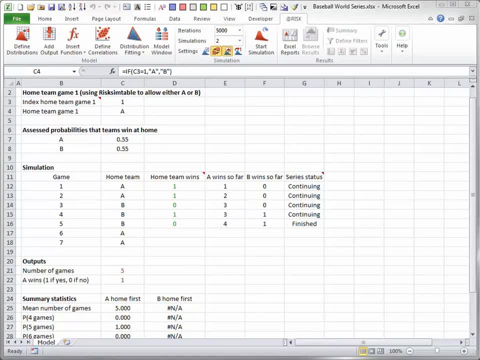 The if functions in column C indicate that the team with initial home field advantage is the home team in games 1,, 2,, 6, and 7. The other team is then the home team in games 3,, 4, and 5.. 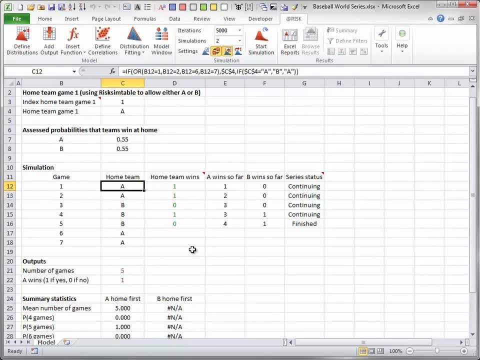 The only random values are the 0, 1 values in column D. Each uses a risk binomial function with one trial and a probability of success looked up from rows 7 and 8.. Values are definitely generated for the first four games, but beyond that they are generated. 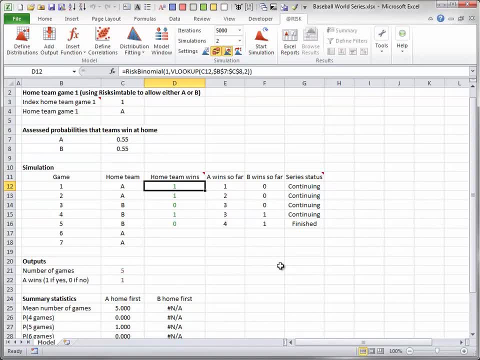 only if the series is continuing. Blanks are entered if the series is already over. This general if logic for games 5 to 7 is used in other columns as well. The first four games are generated only if the series is continuing. The blanks are entered if the series is already over. 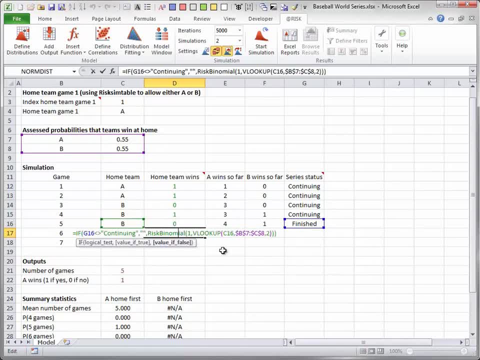 This general if logic for games 5 to 7 is used in other columns as well. Columns E and F capture the cumulative number of wins for each team. This is done for team A in column E with nested if functions. Then it is done for team B in column F by using the fact that the two teams' wins must. 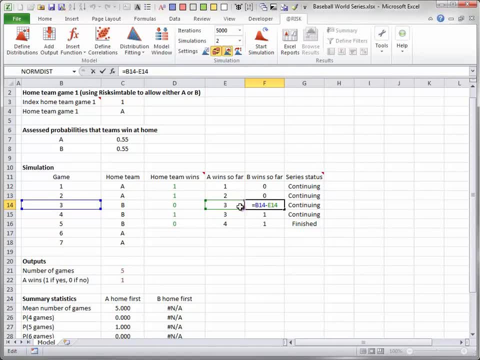 sum to the number of games played. Finally, Column G tells the status of the series. It is definitely continuing after games 1, 2 and 3.. After that it depends on whether either team has won four games The first time this happens. Column G records finished. 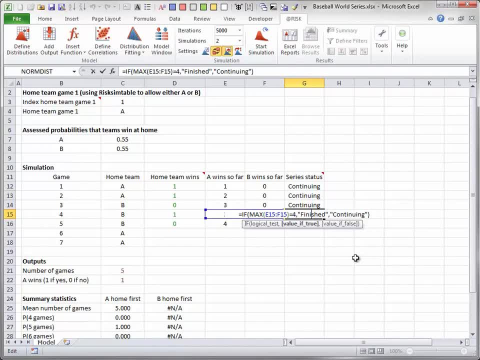 After this it records blank. I will press the F9 key a few times to illustrate how the World Series might play out. Two cells have been designated as at-risk output cells. In cell C21, the number of games played is the number of non-black entries in column. 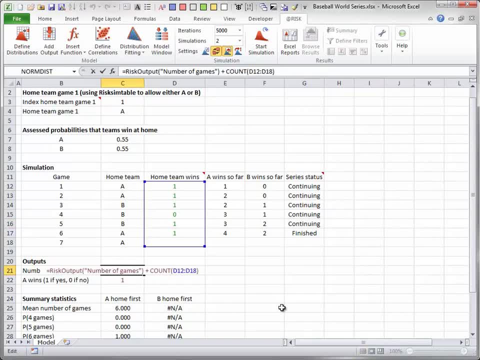 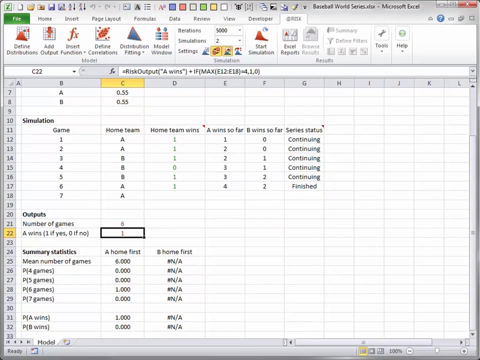 D In cell C22, Team A is the winner if the maximum value in column E is 4. Then a number of at-risk statistical functions can be used to find summary statistics on the length of the series and the winner, Because two simulations are run, one for each possible team. 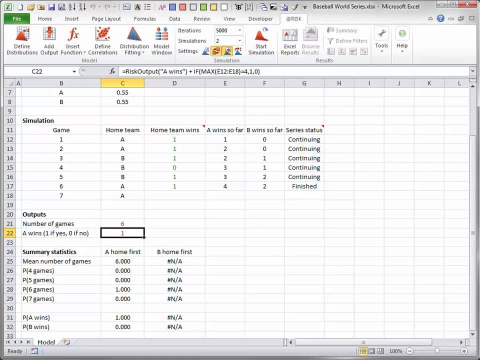 with first home field advantage. each statistical function has last argument 1 or 2.. Note how the probability that a series has exactly, say, 6 games is calculated. It is the probability of less than or equal to 6, minus the probability of less than or.